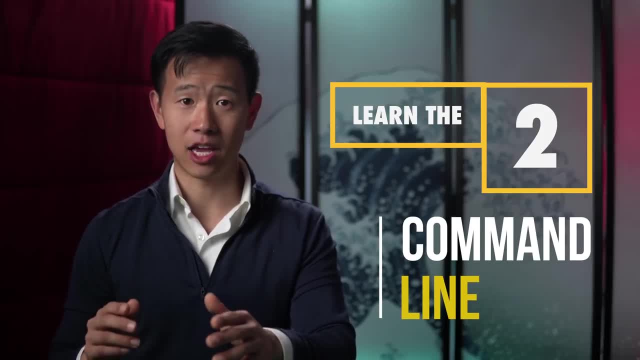 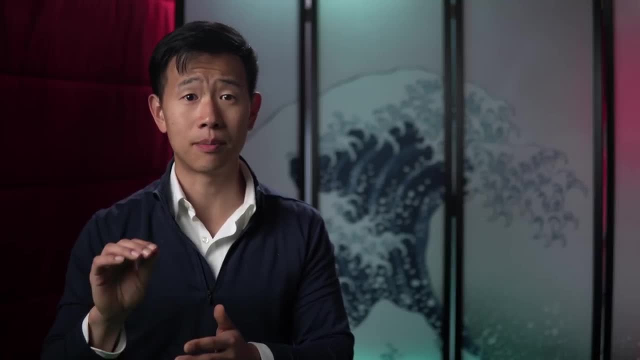 Moving on to number two, Learn the command line. Don't run away, but embrace it. The command line interface, commonly referred to as a shell, is the simplest and arguably the most efficient way to interact with an operating system. For example, if I'm looking for an entry in this CSV file, 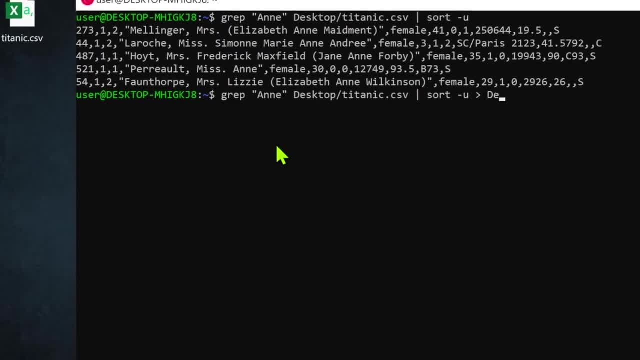 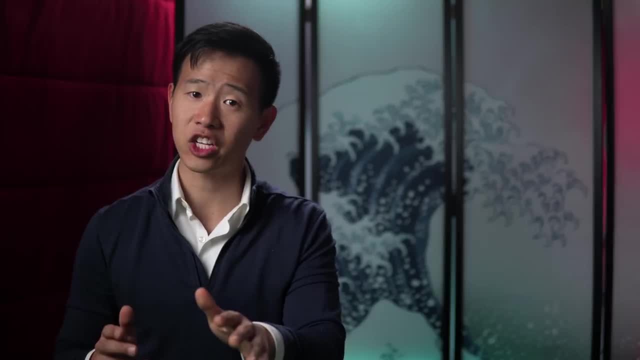 Excel might freeze or crash. Running a lightweight shell command gets me what I need in no time. Why is it called a shell? The important parts of an OS that actually make it run is called the kernel, because it functions at the center of the system. 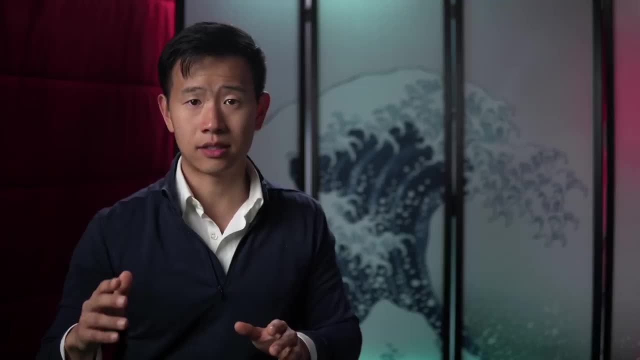 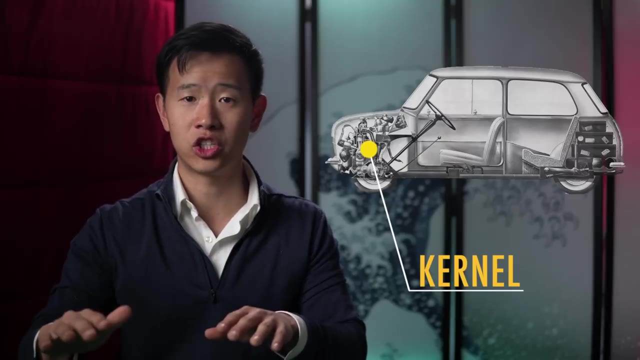 The part that's exposed to a user is called the shell, since it wraps around the kernel. It's just like a car where the steering wheels, pedals and dashboards- giving you control over the engine or transmission- all exist in the shell of the car. 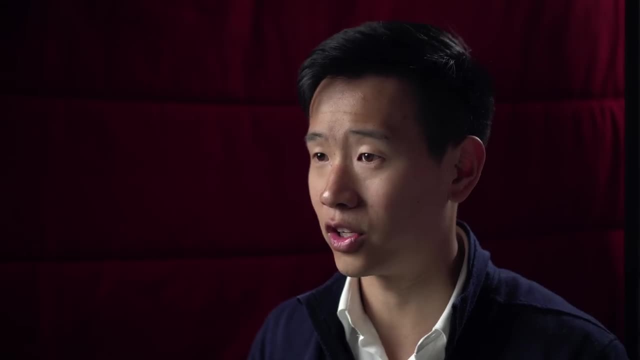 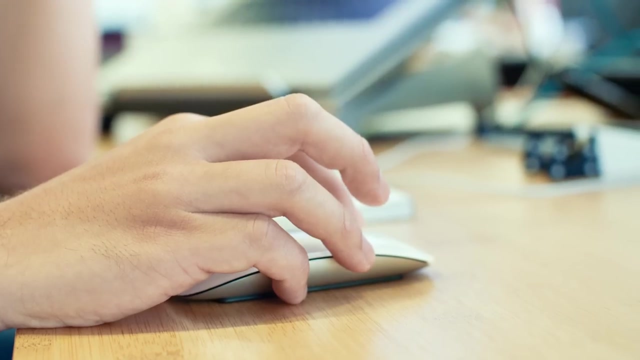 The command line gives you the lowest level access to software functionality that comes with an operating system. Many of the most useful tools don't have a graphical interface to point and click. Mastering the command line expands your arsenal and lets you get more done with less. 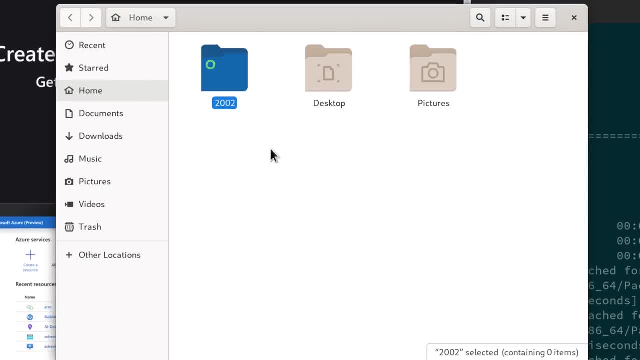 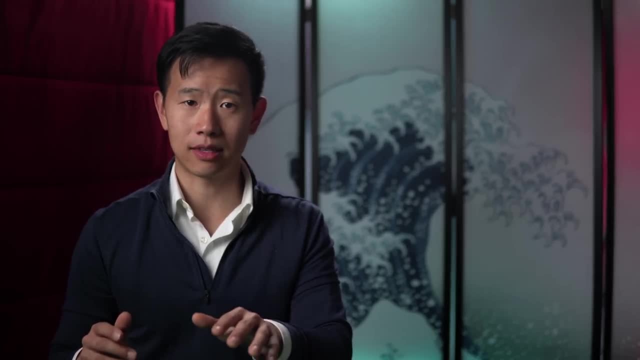 It lets you be able to use scripting and automation to tackle repetitive tasks that would otherwise waste lots of time. Automating your workflow by learning the command line makes you a tremendously valuable asset to the team. I recommend starting out with Bash or Born Again Shell, since it comes default with almost every Linux distribution. 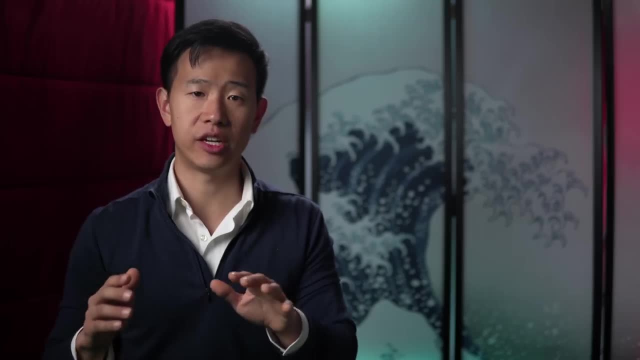 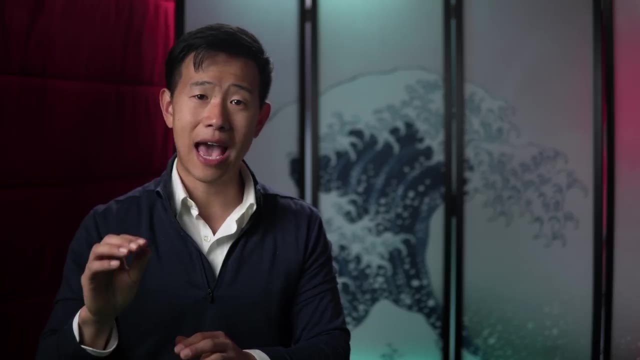 macOS used it in its terminal app, but has since changed to Zeesh or Zeeshell and has some nicer features. If Bash is like a Toyota, then Zeesh is more like a Lexus. Bash is so popular and effective that Microsoft actually released the Windows subsystem for Linux. 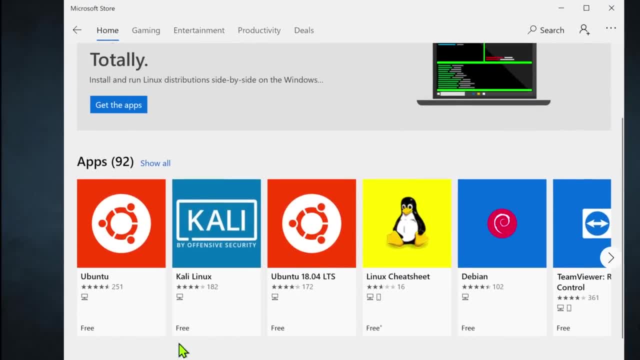 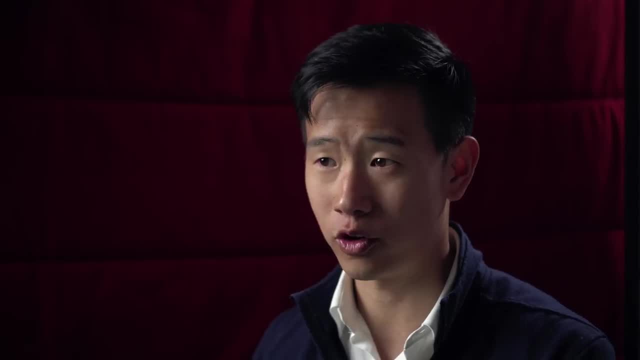 or WSL, and lets you install several different Linux flavors to use Bash as a native app. This is super convenient, since I can access all of my Linux tools without having to switch to a virtual machine. Now understand that PowerShell is actually the go-to native shell for Windows. 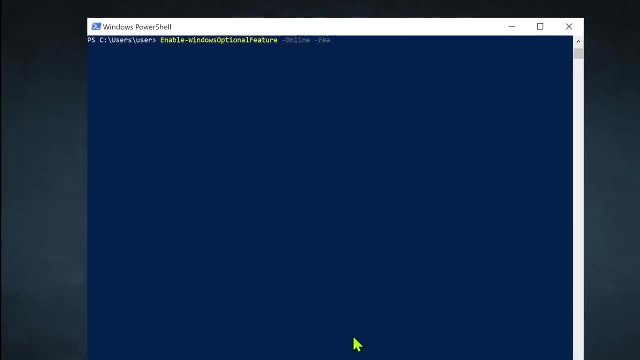 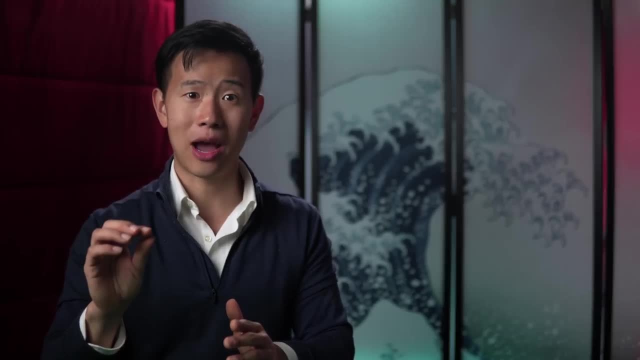 It's very different from how you would use the Linux command line, but gives you a ton of powerful Windows administration abilities. If you work in an environment where Windows is the primary OS, definitely learn PowerShell as well. I'm going to start a series on the Linux command line very soon. 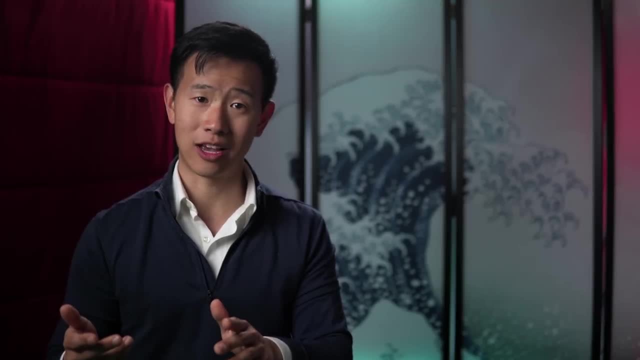 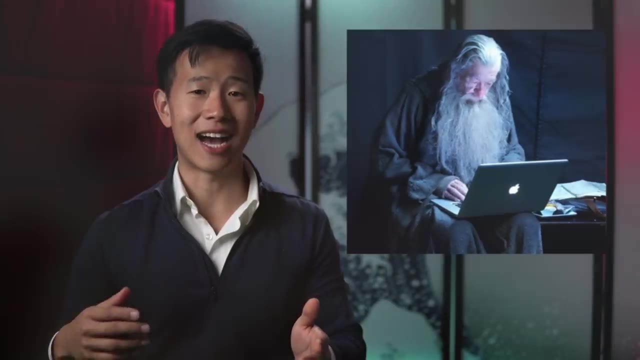 Comment below to let me know what tools and concepts you'd like to learn. System Administration- All of us with a computer or smartphone- from your grandma to IT wizard- is really a sysadmin at some level. It all depends on what level you're at. 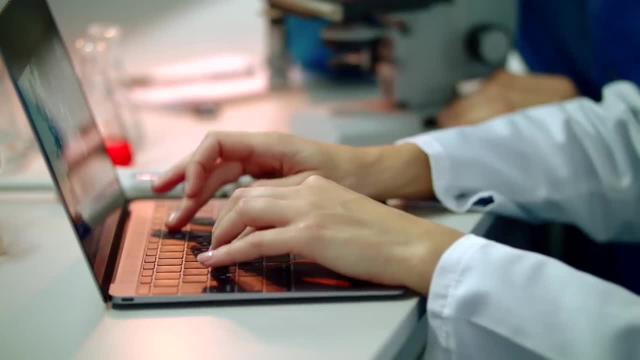 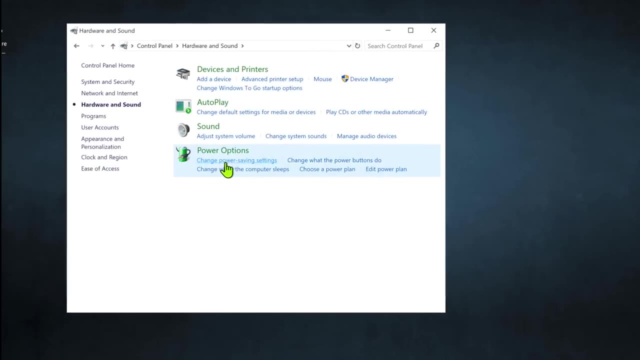 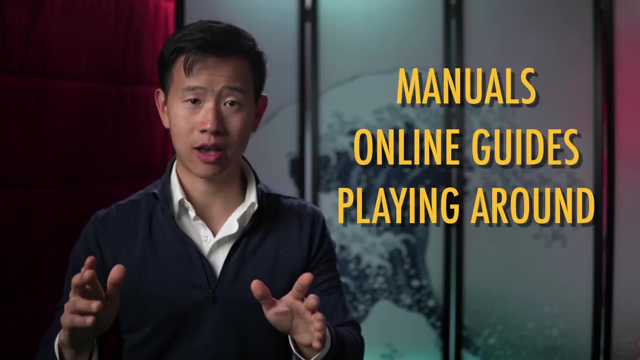 System administration involves the configuring and maintaining of computers, whether a personal device or a high-powered server. When I was first using computers as a kid, I loved to dive down into every single setting available on the computer just to see what it did. Reading manuals, online guides and playing around just drove this curiosity further. 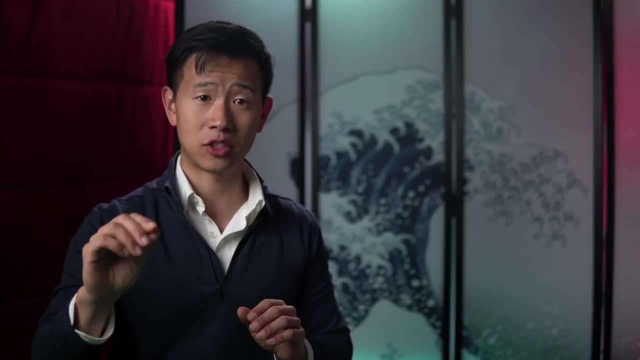 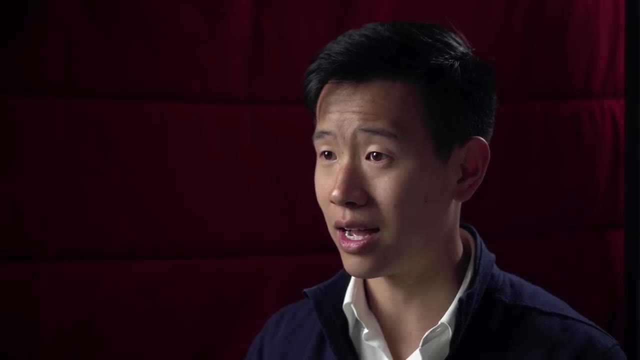 By doing that, I became the family IT help desk System Administration. System administration is about knowing your platform and various tools inside and out to be able to help others who don't. Whatever your skill, I challenge you to fiddle around and learn by doing. 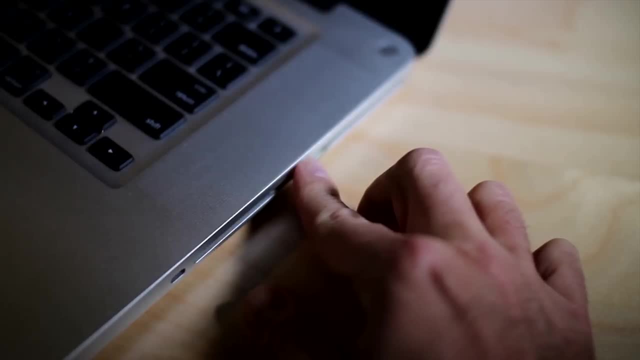 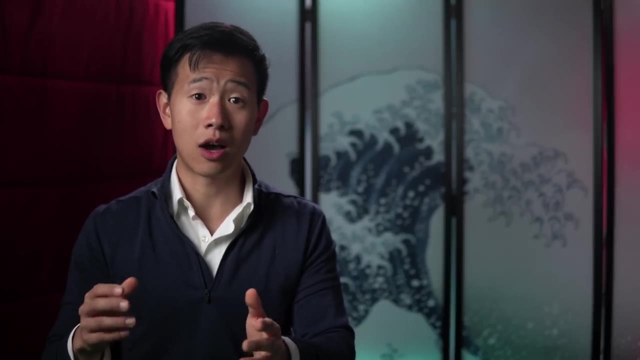 Delete some files and try to recover them. Download, open and monitor old viruses in a virtual machine with tools like Windows Sysinternals to see what they do. Try to extract files and passwords off a computer without knowing the login info, Whatever it is. push the limits of what you already know by reading guides out there. 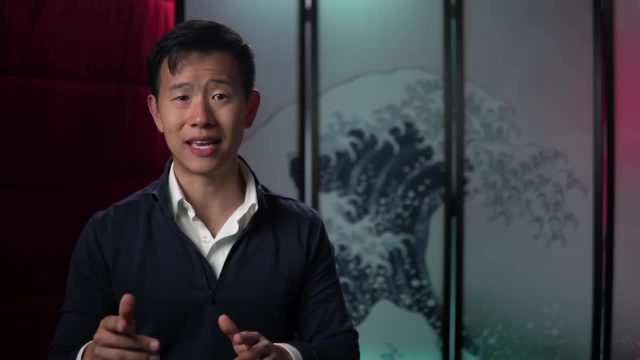 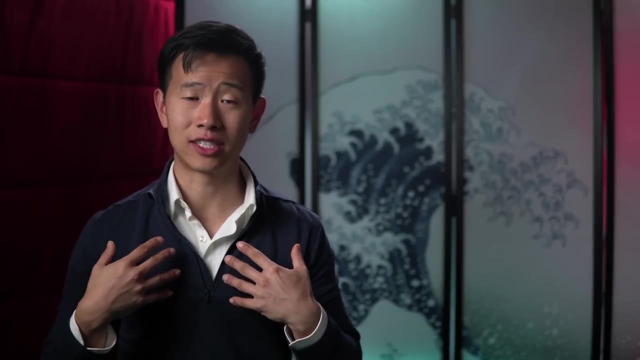 and following along. Practice a little more each day and you'll get there. You'll level up in no time. Number Four: Computer Networking. This is the heart and soul of it all, What I like to call the cyberspatial laws of physics. 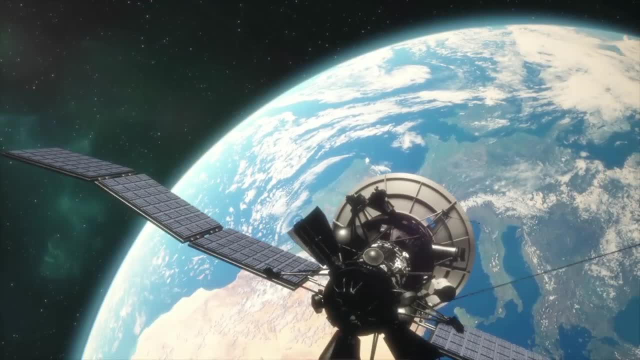 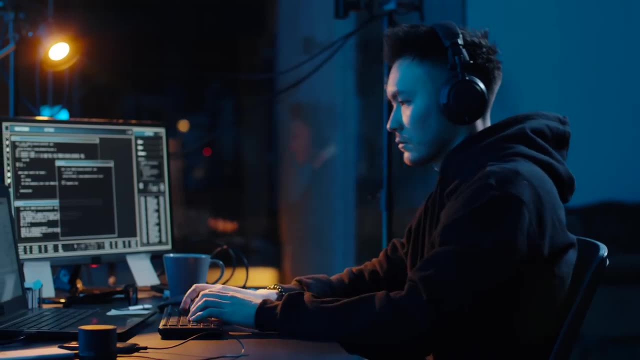 It's understanding how devices interact with each other and how data gets from point A to point B. A strong foundation in networking will make you a rock star troubleshooter, whether you're red teaming, defending or running day-to-day IT ops. 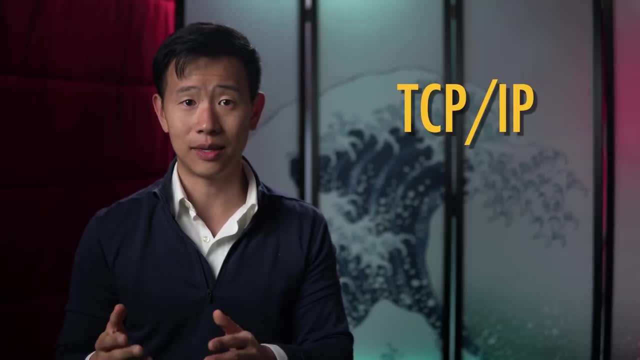 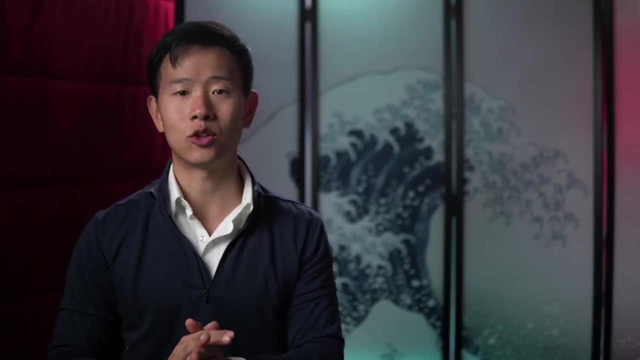 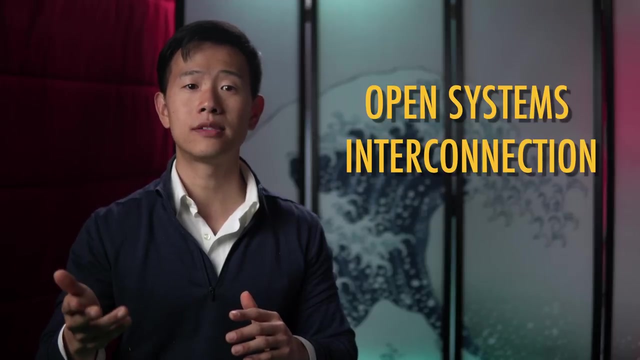 There's two conceptual models that govern computer networking: TCPIP and OSI. They group all your different networking and telecommunications protocols into layers. TCPIP is older and uses four layers: Network access, internet transport and application layers. OSI stands for the Open System Interconnection. 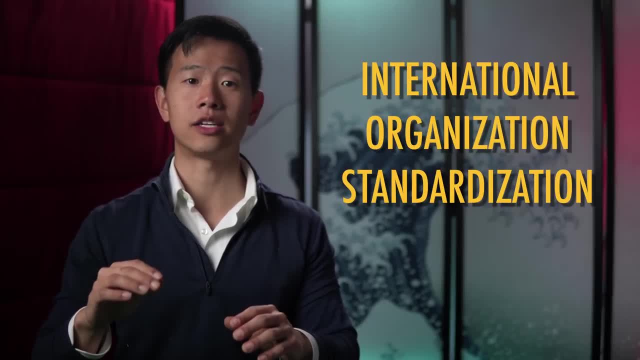 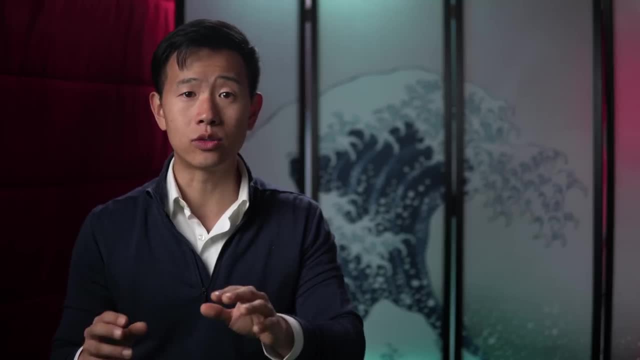 which is developed by the International Organization for Standardization, or ISO. These guys define everything from country codes to time and date formats. OSI is newer and uses seven layers: Physical data, link, network, transport, session, presentation and application layers. 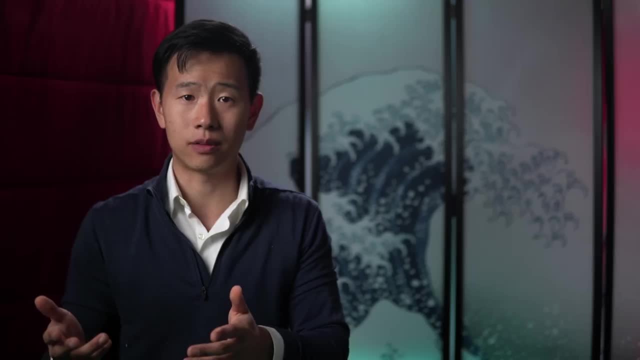 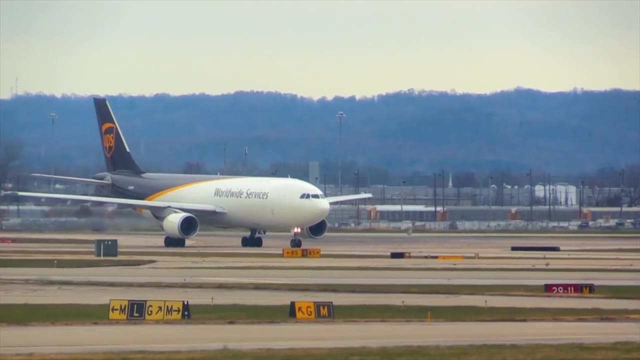 All these layers are just a one-time thing. It's not a way to describe what's happening where. So if you're receiving a package from someone in a different country, it's going to get passed between envelopes, boxes, vehicles and planes.